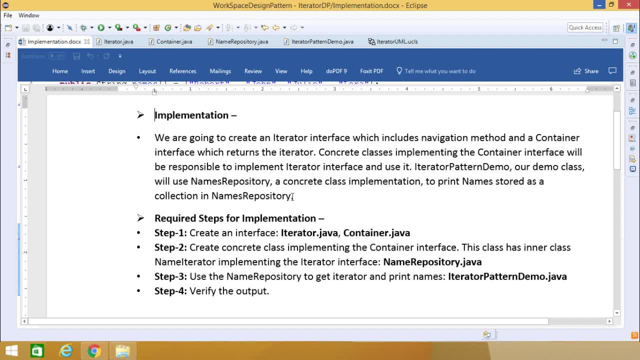 example, we are going to create an iterator interface which includes a navigation method and container interface which returns the iterator. Concrete classes implementing the container interface will be responsible to implement iterator interface and use it. Whoa wait, let me tell you the structure of the experiment program. Iiterator pattern demo. Iterator pattern demo obtains 3합니다, inspiring bachelor pass and final search, etc. which help to analyze the problem in no break square in time. to make it easier, One of the commands for this implementation is use of Meltoney set Democrat. So now I have to take in the phrase seck新ander. 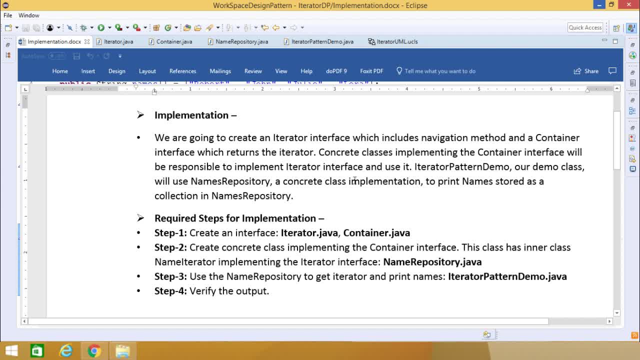 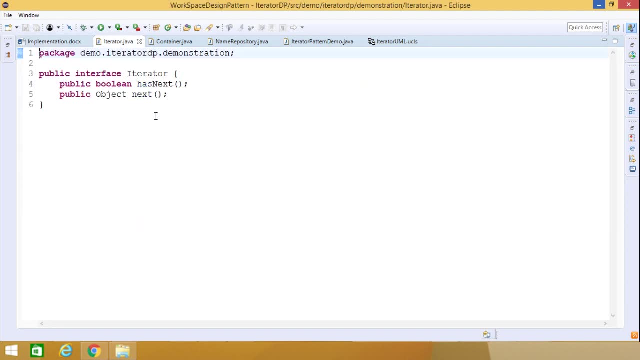 demo class and will use name repository- a concrete class implementation, to print names stored as a collection in names repository. so let us go for the implementation step by step. step one: create an interface, iteratorjava and containerjava. so here we are having this iteratorjava, which is having the prime navigation methods are there, and we are having this containerjava. 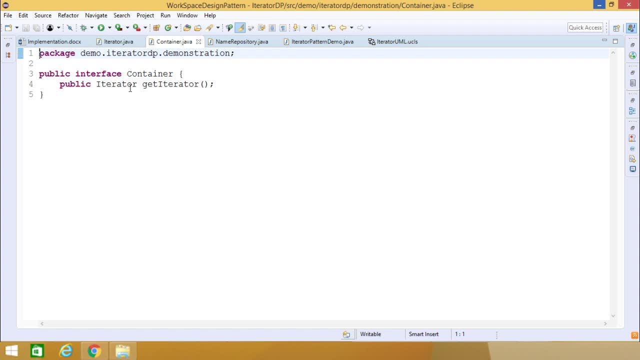 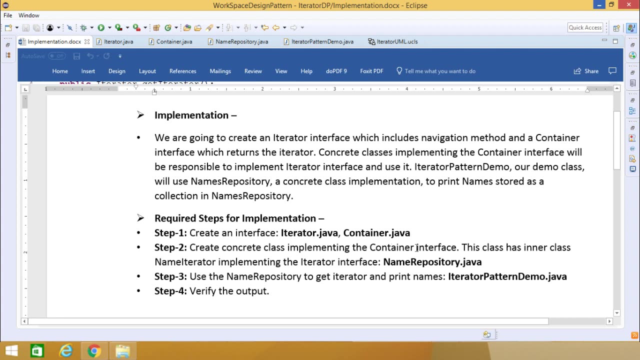 which is having this get iterator- unimplemented method, which returns iterator object. now we are going for the step number two: create concrete class implementing the container interface. this class is also having one inner class, known as the named as named iterator: name iterator implementing the iterated interface, and its name will be name repositoryjava. 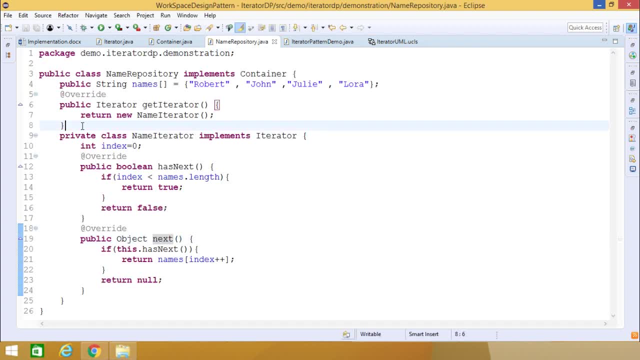 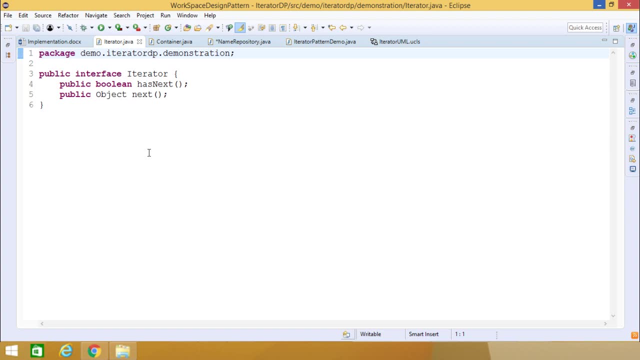 so whatever we have planned that has got implemented here you can find that we are having this name. iterator is the inner class which implements this iterator interface. we know that in case of iterator we have we had two navigation methods. one is the hash has. next, another one is: 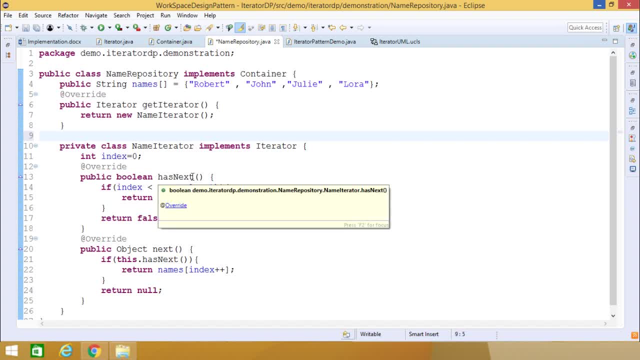 the next. so they have got implemented here, so has. next is checking the value of index. index was initially initialized with zero. with this names dot length, we know that names dot length is nothing but here four, because we are having four names. are there in this names string array? then it will. 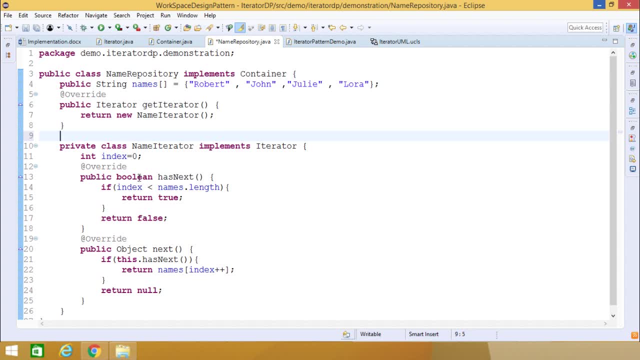 return true, otherwise it will return false. so has: next will return boolean, and that was mentioned in this iterator dot java interface. and here we are having this next function which returns the object as output and this dot has next: if it is true, then names index plus plus will be returned. 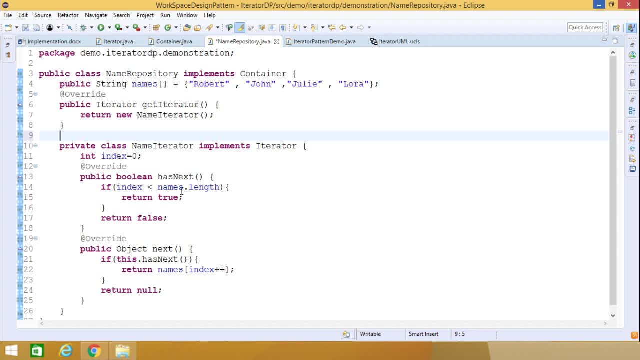 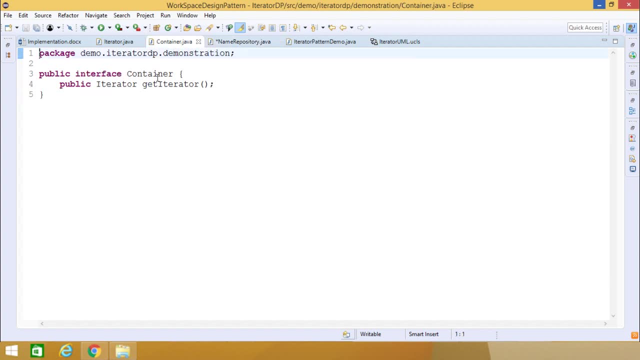 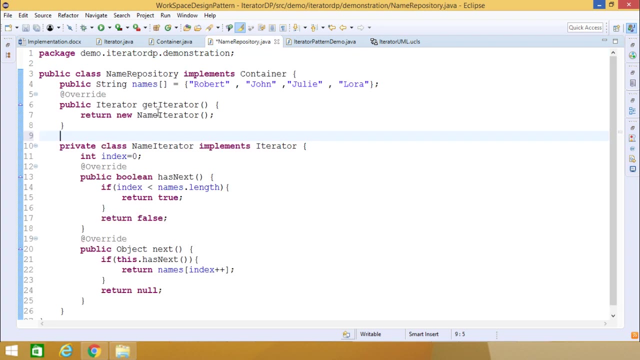 otherwise none will be, none will be returned, and that is our name iterator, that is the inner class. this name repository is actually implementing this container. so we know that container is the interface which is having a only one method, that is, the get iterator, which returns iterator objects. so as a result of that, 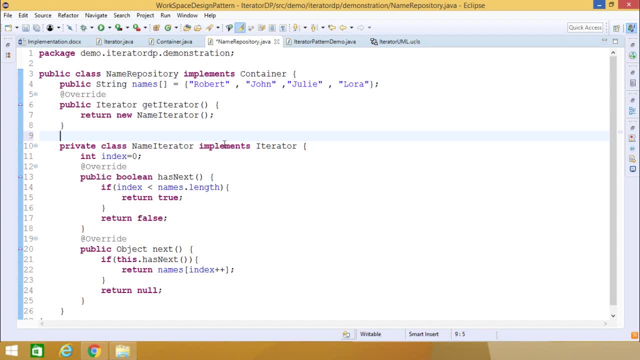 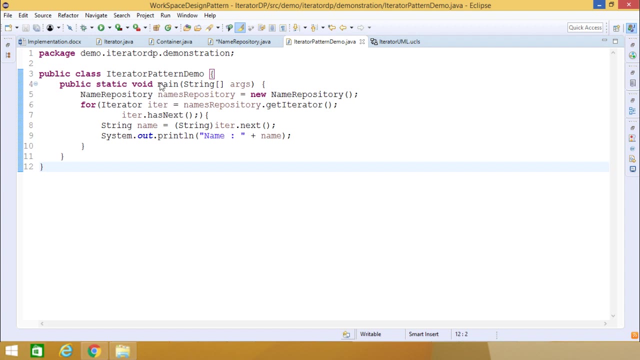 we are going for return new name iterator. name iterator implements iterator so it can easily be written. so we are going to create one name iterator class object name iterator is the inner class. so last, at last, we are going for this iterator pattern demo. you can find that in case 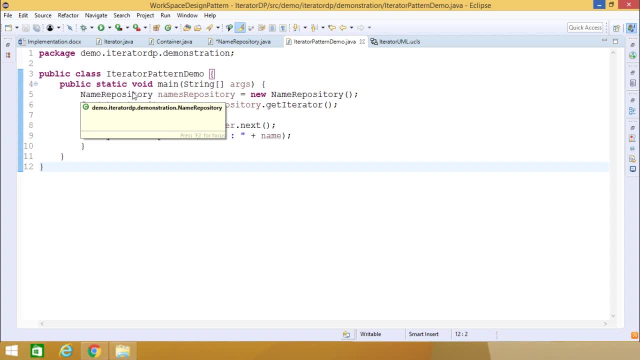 of iterator pattern demo. we are implementing or we are just defining one object under the name repository class and then we are going for for iterator iter is equal to name repository dot get iterator. we know that get iterator returns one iterator class object and this particular initialization will be done until this iterator dot has next returns true and then string name. 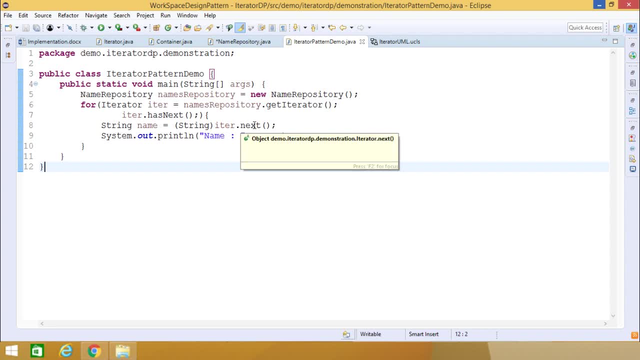 is equal to, so iterator dot. next, you know that in case of iterator dot, next we're having this one. so this is the name repository class object. and then we are going for for iterator. iter is equal to name. next returns object. so we have done the type casting string type which has been assigned to. 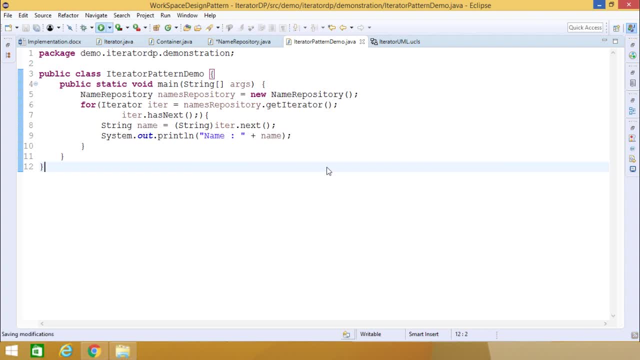 name and name has got printed. so if we execute this code here, we are getting this respective names, which has got retrieved from the this, that is the name array, string array, and then through this iterator they have got printed, and with the using the function that is iterator dot next. 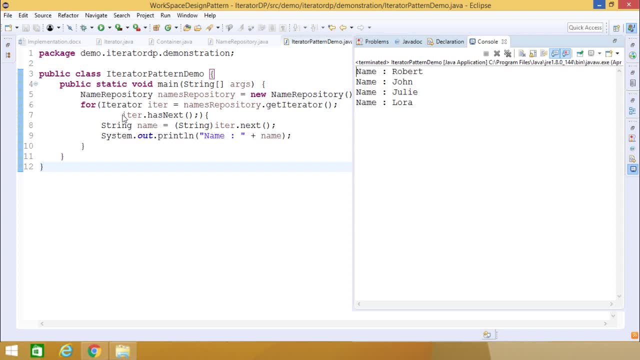 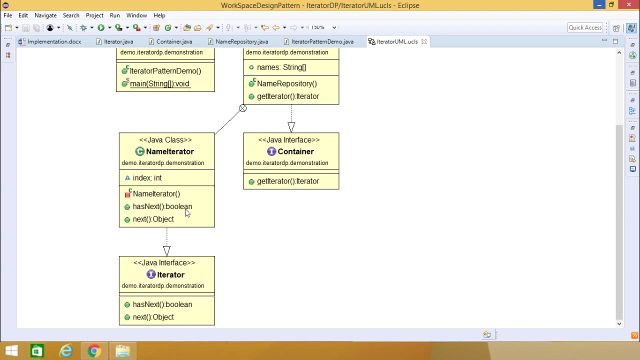 and this particular for loop will be executing when iterator dot has next will be returning true. so we have shown you that, how this code has got coded, and now we are going for the class diagram. so this is our class diagram. iterator interface is there which has got implemented in name iterator. 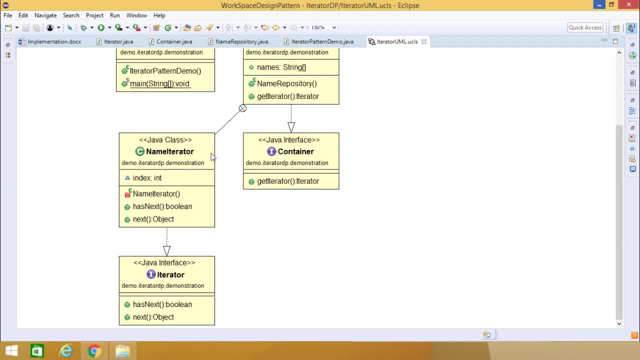 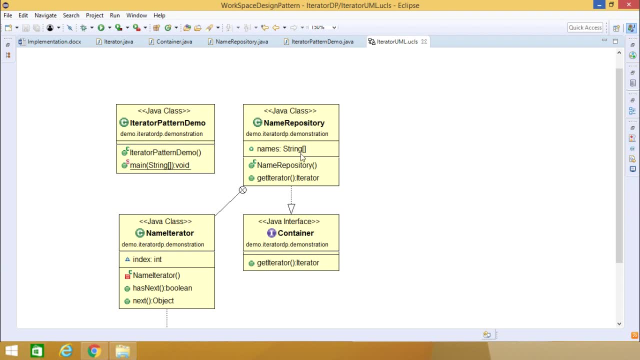 this iterator has got implemented in name iterator and this name iterator is nothing but one inner class, which is nothing but one inner class of this name repository which is having a this names as a string array and name repository is the constructor. we are having this get iterator and this particular get iterator you can go to. 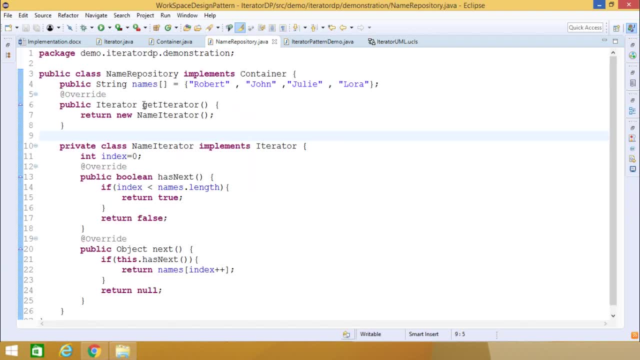 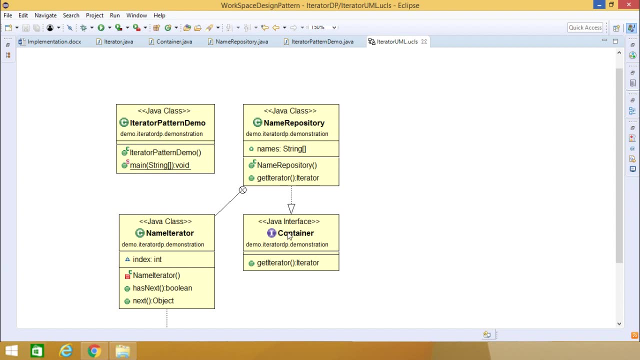 the name repository so you can find this one. there is a get iterator is a method and this name repository is implementing container, so that's why we are getting this implementation here. so container is nothing but one Java interface, having got only one unimplemented method, get iterator, which returns iterator name. 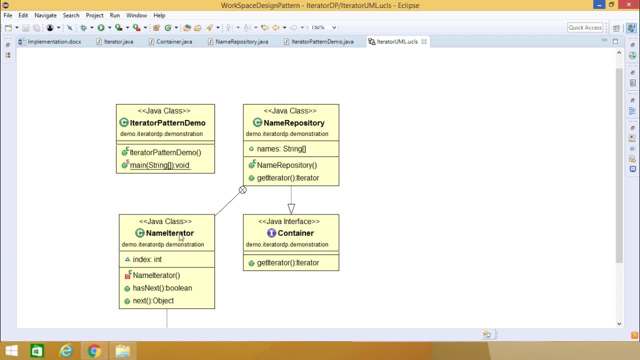 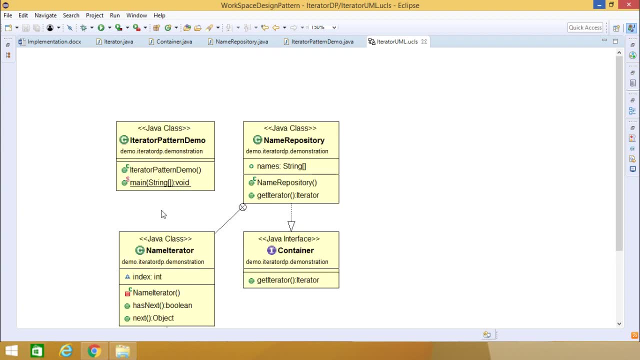 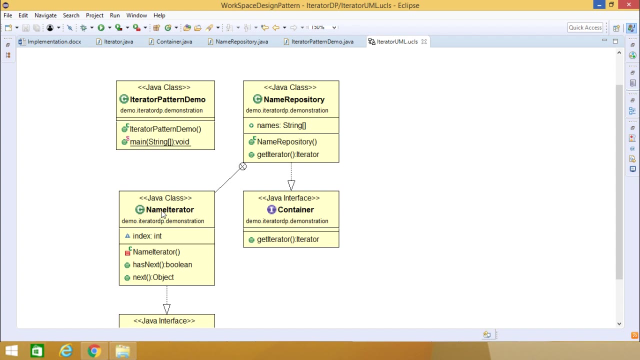 iterator is the inner class of this name repository name. iterator is implementing iterator interface and this is our iterator pattern demo class. so in this way, in this particular demonstration, we have discussed how this iterator design pattern can get implemented using Java code. thanks for watching this video. 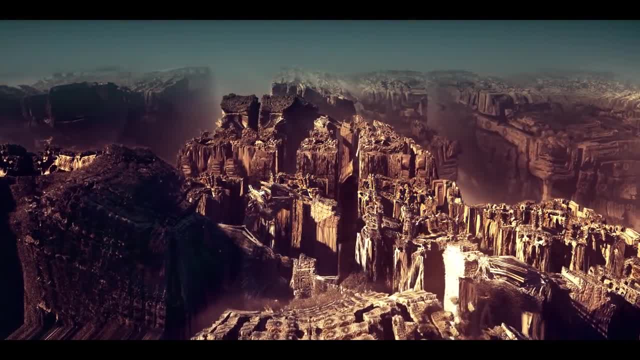 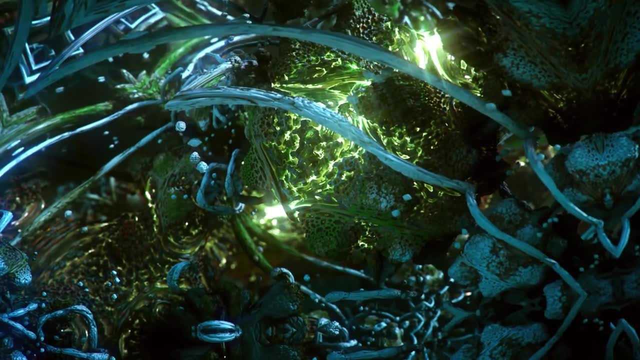 This is Julius Horshuis, the fractal guy. Maybe you've seen some of my work. I'll show you some here. I just wanted to show you some examples of settings in formulas and what kind of effect they have on the world. 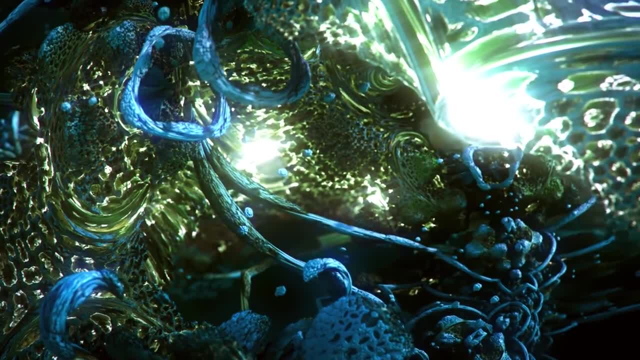 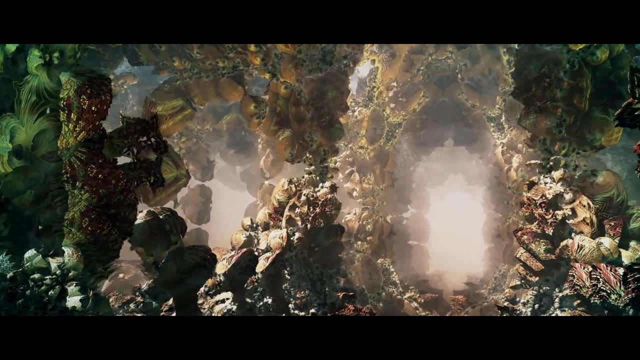 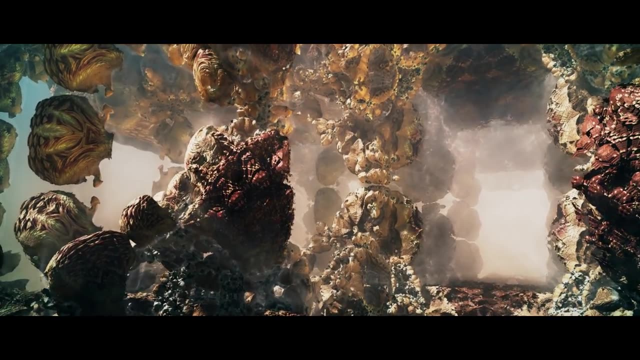 It's a pretty crazy world out there in the fractal landscape. so I just thought, maybe a relaxing time by looking at some of the parameters in the formulas, and we'll look at some fractal architecture as well. I will say I am not a mathematician and I don't understand anything.